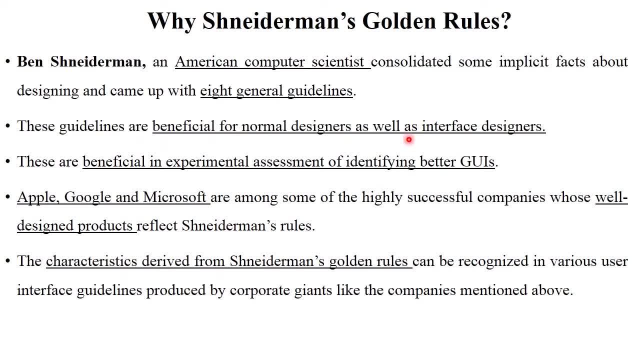 These guidelines are beneficial for normal designers as well as interface designers. These are beneficially in experimental assessment of identifying better GUI. GUI means Graphical User Interface. You should make up quality, fill or usable graphical user interface of the particular application or the particular product. 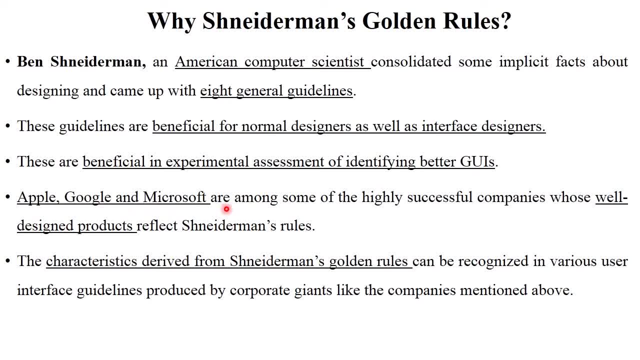 There are different companies Like Apple, Google, Microsoft, Microsoft are among some of the highly successful companies which well design and produce reflect Schneiderman's rules. The characteristics derived from Schneiderman's golden rules can be recognized in various user interface guidelines produced by corporate giants like the companies mentioned above. 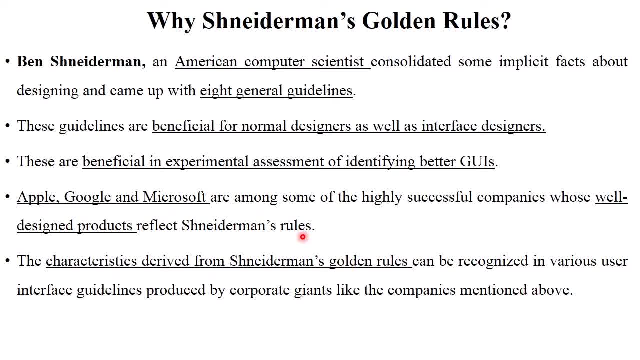 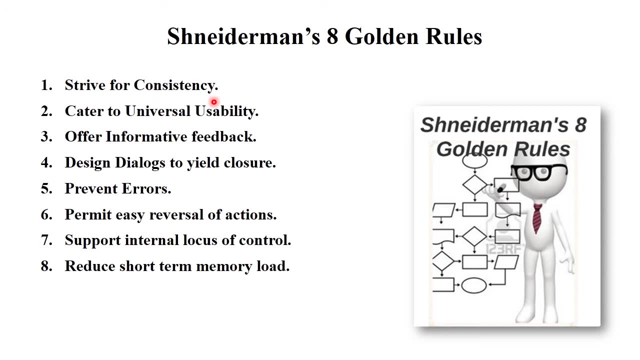 So, simply, these all eight golden rules are followed by each and every designer to design a particular software or a particular application. clear, Next, Now see here. these are the main eight Schneiderman's golden rules. The first: strive for consistency. cater to universal usability. next, offer: informative. 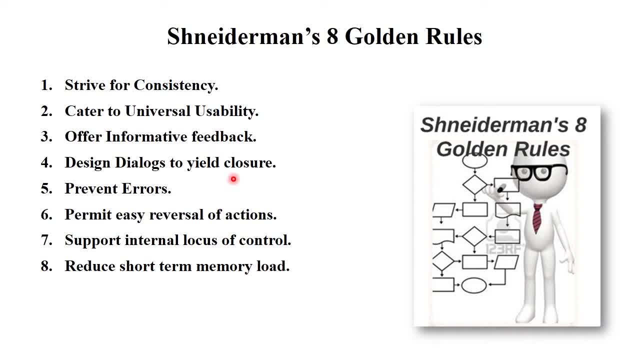 feedback. next, design dialogue to yield closure, prevent errors, permit easy reversal of action, support internal locus of control and reduce shortcomings. So these are the eight golden rules of Schneiderman's which will be useful for each and every designer to generate quality product or quality design clear. 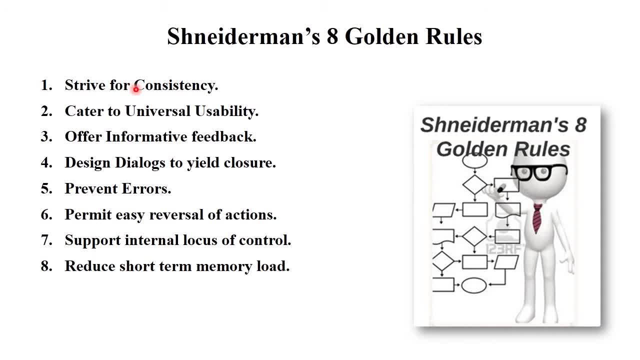 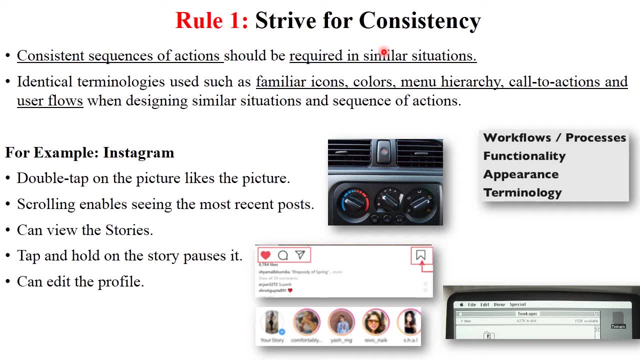 So let's see one by one. The first rule is strive for consistency. next. So what is mean by strive for consistency? We all are familiar with the word consistency. Consistent means constant right, So consistency means consistency, So consistent sequence of actions should be required in similar situation. 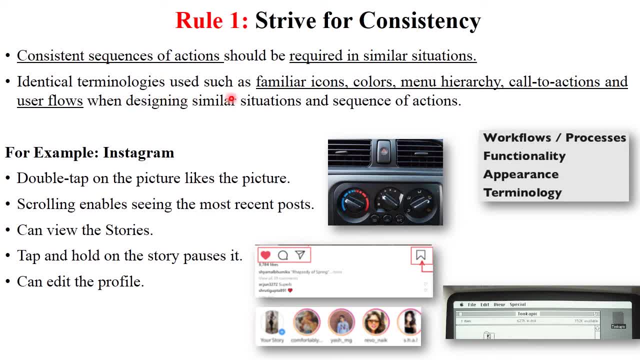 There are some identical technology used, such as familiar icons, colors, menu, call to action and also user flow while designing a particular situation or sequence of action. For example, see here: We all are familiar with Instagram, right? So double tap means picture. like the pictures, right? 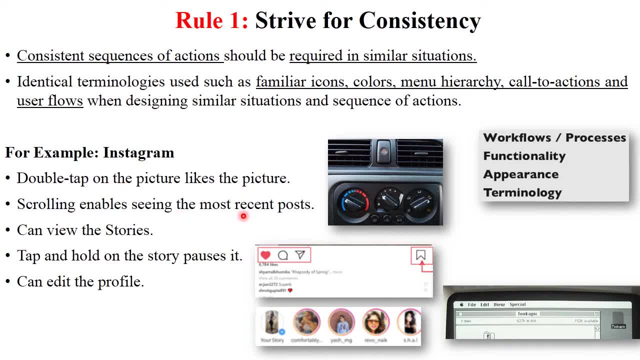 Scrolling means enables seeing most recent post. We can view it right. So double tap means picture, like the pictures right. Scrolling means enables seeing most recent post. we can view the stories. tap and hold on story pause it. we can edit the profile right. so these 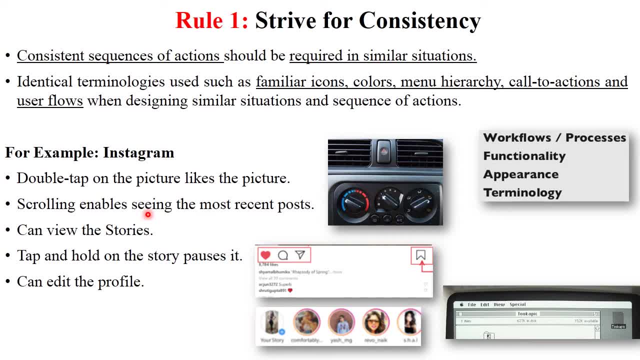 are the examples. that is consistent features. these features similarly available in other social medias like whatsapp. facebook also used. this kind of features means these are the consistent features, or constant features. users are most familiar with that right again. next example is in microsoft word, in notepad or in microsoft powerpoint, there is file edit view. this kind of options are available. 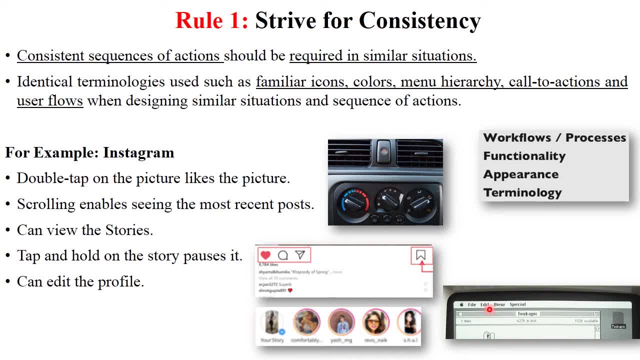 these are the most common features. users easily used the particular application. that are the consistent features. right, so this is the concept of style for consistency. it includes workflow, different functionality, appearances, terminology which used in similar situation and in sequence of actions. right, so this is the concept of consistency. you should implement it while designing a particular product. 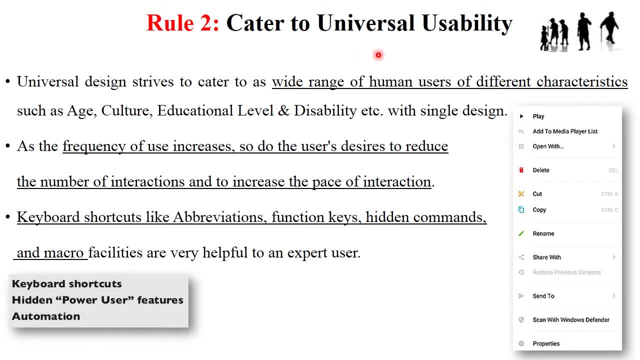 next. the next rule is cater to universal usability. universal designs strive to wide range of human users of different characteristics. right, there are different types of users are present: their age, culture, educational level and disability, etc. so while designing a particular product, you should consider regular information, including basic steps like aspect and weight. what so ever develop. 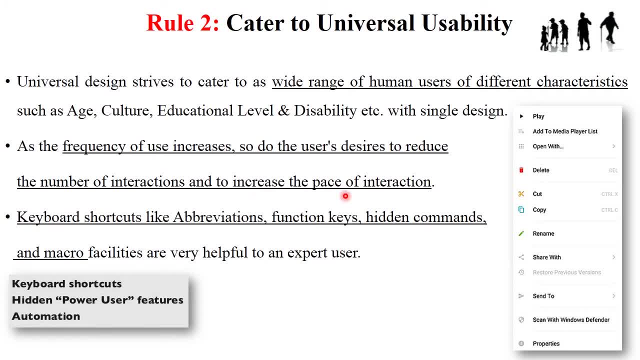 things there are: frequency of use increase and show the user's desire to reduce number of interaction and increase the pace of interaction. the simple way- another simple way- that is always use keyboard shortcuts like abbreviation function, key, hidden commands, macro facility are very helpful to an expert users, right. so design a particular software by using the shortcut key, for example, cut control. 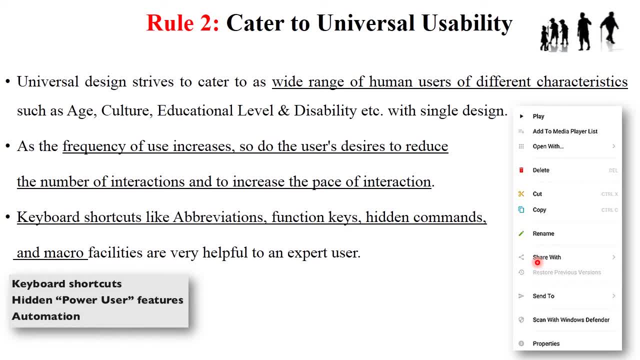 copy control c, then paste control v. right, we all are used with shortcut keys, so always design a particular software by analyzing all those things so cutter to universal usability. this principle includes keyboard shortcuts, hidden power user features and some automation things. right, so you should design this, all things while designing a particular product. clear next. 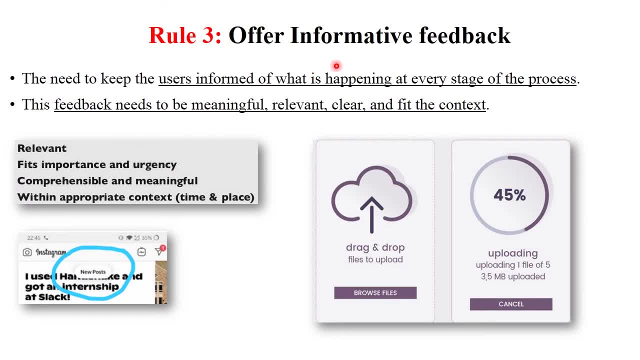 text. and third one is offer informative feedback: the need to keep the users inform what is happening at every stage of the process. this feedback needs to be meaningful, relevant, clear and fit the context. while designing a particular software, you should provide an informative feedback to the user. see in this diagram. this is the example of Instagram right, the new post. 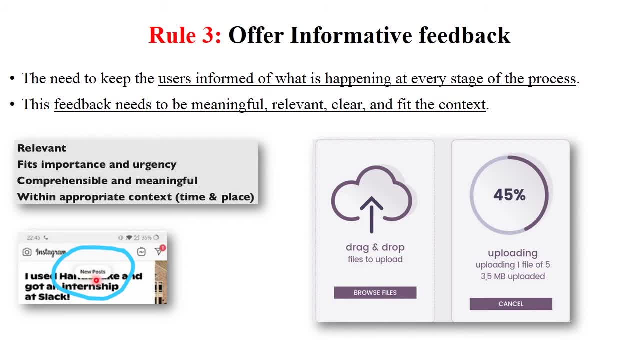 this notice is the example of Instagram. right the new post. this notice is the example of Instagram. the notification of pop-up notification will be generated right, so it gives the proper feedback: feedback. then there will be a new post will be uploaded. clear. the next example: drag and. 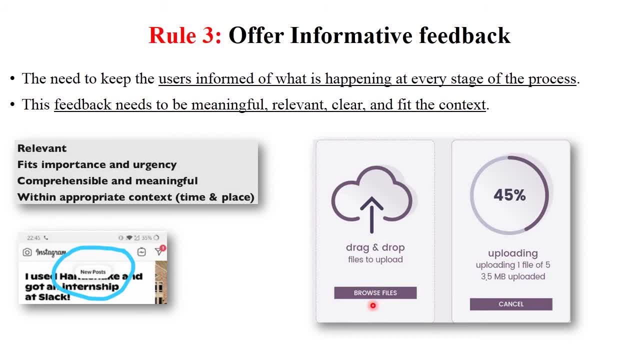 drop files to upload so users may bank that exactly down here right next uploading. uploading a file means user know that what is happening. that is, 45% will be completed and remaining right. so this is just informative feedback. user knows that what exactly happening. so this principle includes some relevant features. 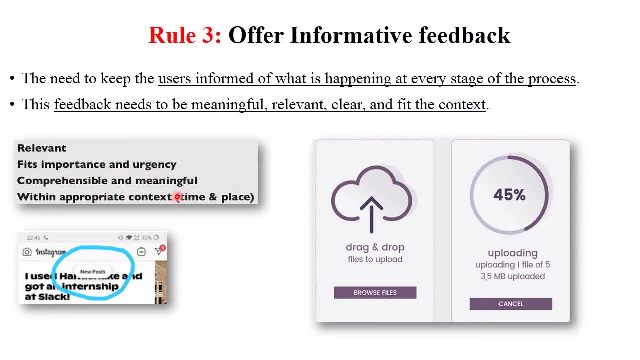 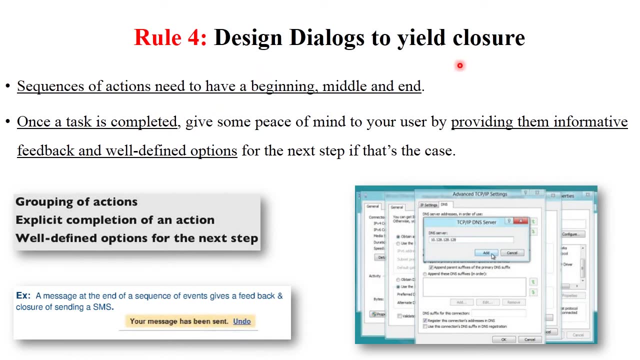 importance and urgency, compressible and meaningful information and appropriate context right. so while designing a particular product, you should analyze all those things next. the next and fourth rule is design dialogue to end closer. this means that the sequence of actions needs to have beginning, middle and end. once task is completed, it gives a provide. 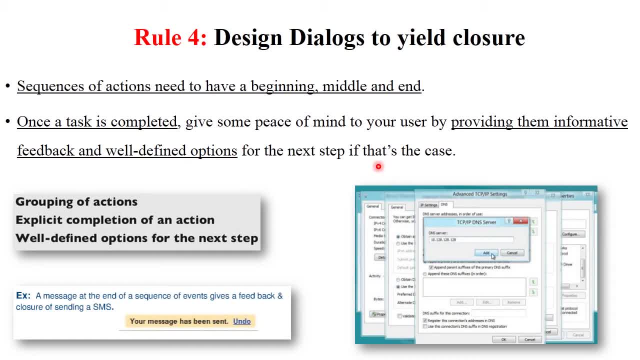 transformative feedback and well-defined options for the next step, right. for example, see here: If you sent a particular message, if you should send a particular email, so there will be a pop-up notification that your message has been sent right. so this is the particular informative feedback and communication. 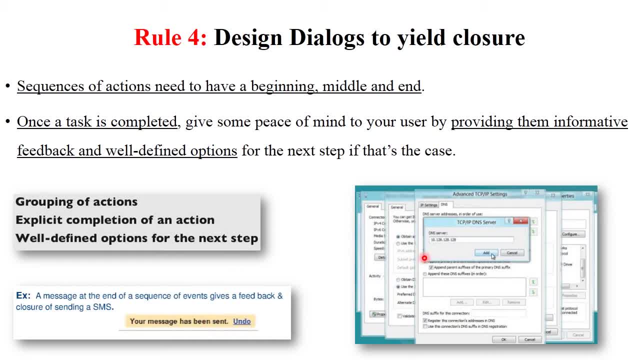 the user and the system, right. the next example is suppose you have to install a particular software. there were some instructions you should press on next, next, next, options, right. so it gives a proper informative feedback to the user. clear, there is a proper communication between user and the system. so this: 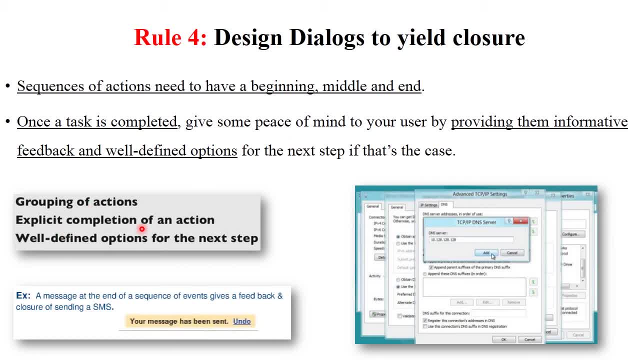 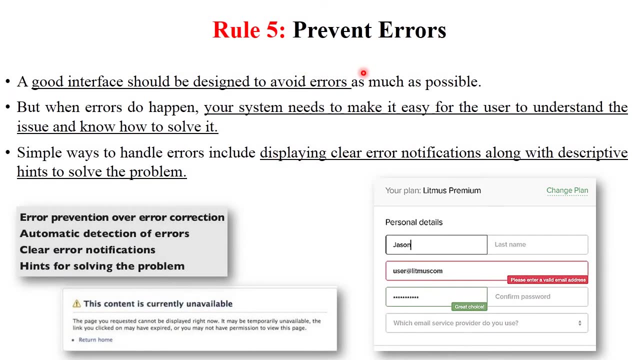 principle includes grouping of action, explicit completion of action and well-defined option for the next step. right, so this is. you should design a particular software according to this way- clear. next. the next rule is prevent errors, one of the most important principle. a good interface should be designed to avoid the errors as much as possible, but when errors do happen, your 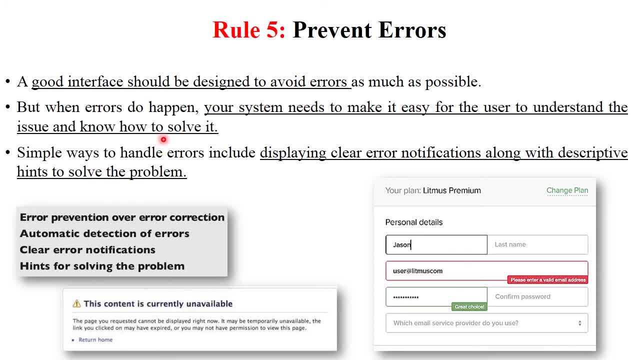 system needs to make it easy for the user to understand the issue and know how to solve it. for example, see in this diagram: suppose you have to enter a particular details in any online form, okay. suppose you enter a raw email address so it gives the notification. or 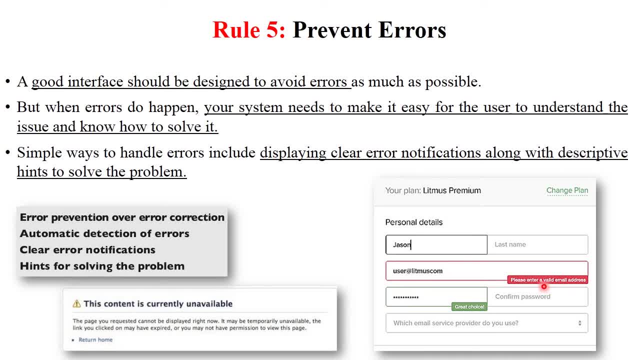 error. please enter a valid email address right. so this is one of the most important thing. users know that. what exactly happening here? clear the next: this content is currently unavailable. this is some particular error message will be displayed clear. so you just take a particular action while show and I'll display this error. 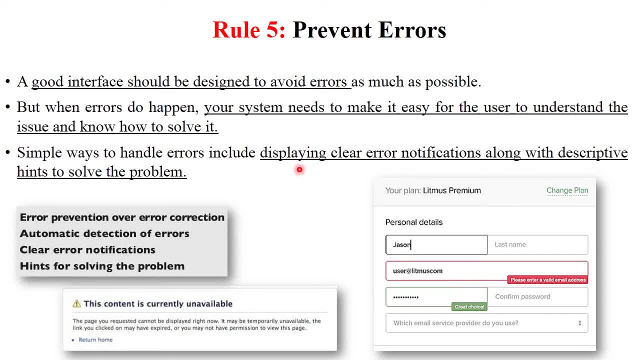 so simple way to handle the errors includes display clear error notification to the user along the descriptive hints to solve the problem right. while entering a password, there will be a hint option clear. so this all things are included in prevent errors. this principle includes error conventions, error corrections, automatic detections of errors. 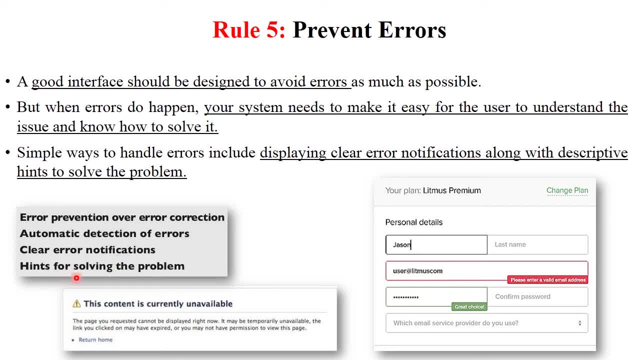 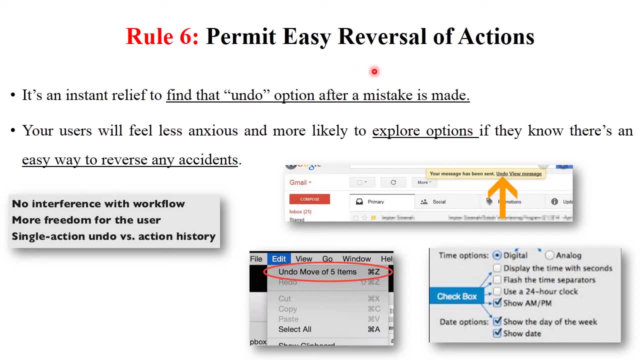 clear error notifications and also there are some hints for solving the problems. so this is your next rule in golden rules. next and the next principle is: permit easy reversal of action. it's an instant relief to find that undo option after a mistake is made we all are familiar with. 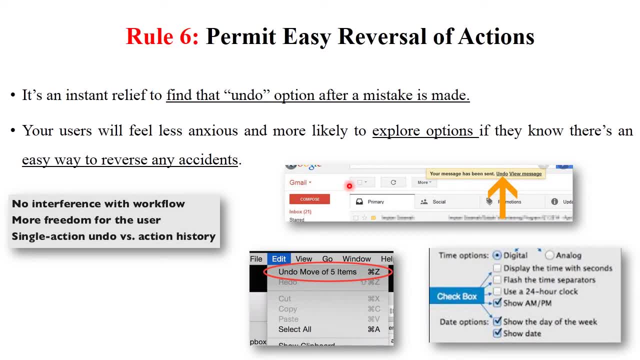 this situation. so you should design a particular software or particular application by giving a undo option. so your users will feel less anxious and more likely to explore options if they know there is an easy way to reverse any accident. so reverse is one of the most important features. 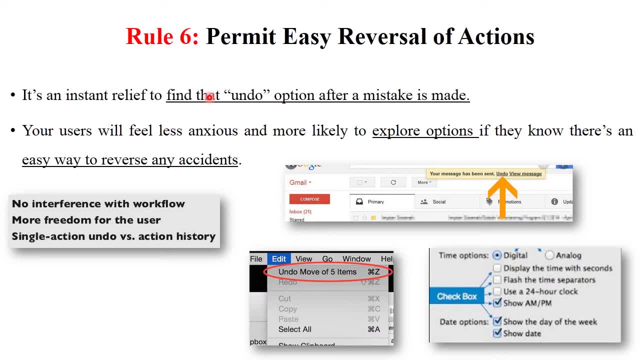 while develop or design a particular software. so these rules includes no interference with workflow, more freedom for the user and single action undo you. this action history clear and these are the some examples. your message has been saying: this pop-up notification will be generated in gmail, right, so there is undo option will be provided again undo. 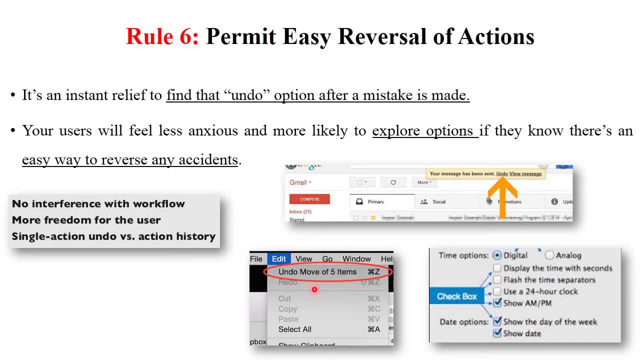 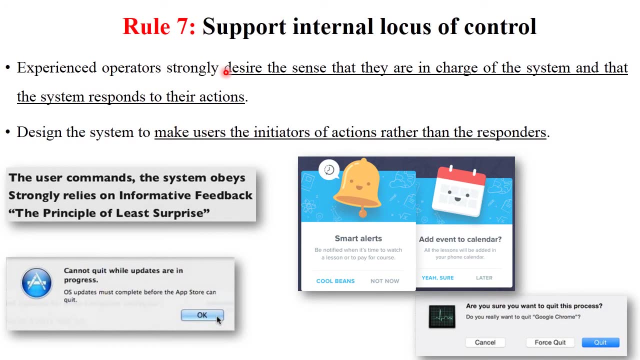 option will be provided in some word file or notepad. right again there are some checkbox and radio buttons will be provided. so users select a particular option as per their opinion or as per their requirements, right next. next rule is support: internal locus of control. experience operators strongly desire the sense that they are in change of the system and that the system respond to their action. design the system to make user the. 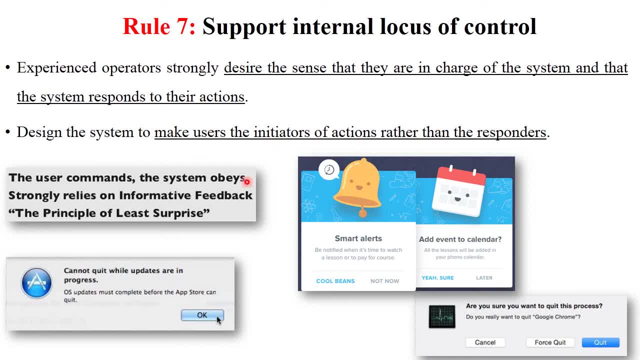 impetus of action rather than the responders. this means that there are particular decisions or particular requirements is taken by the users while use the particular system or the application. see there are some examples. their particular notification will be generated. cannot quit what abbas are in progress. right this notification given by the system, user's not following. 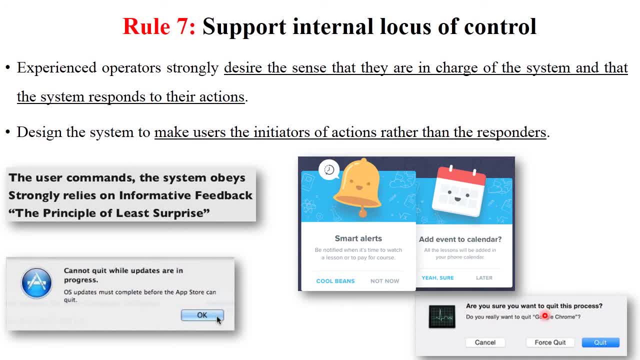 right that there are some notification and reassured. we want to get this process so if expert depends on the user whether it is correct, cancel or force wird except up. so users has a high priority at that time and use this app, blockdale and software time. old Irish has a high priority at that time, toagit io. and officer. again wait a minute. need a list for different versions. user user es். okay, let usatto. if you want you can. as strong commercial interplay이라 whether it is cool housed by the star letter, really clear, while malesges is nothing, but always they are there. 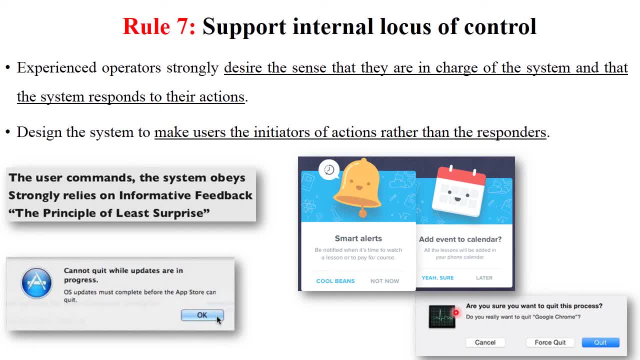 see if they are trained by others, such as answers also, and for let them лет high priority at that time. there are some smart colors. add events to calendars. this kind of option will be given while designing a particular application. so these principles include the user commands the system obeys strongly release on informative feedback, the principle of list. 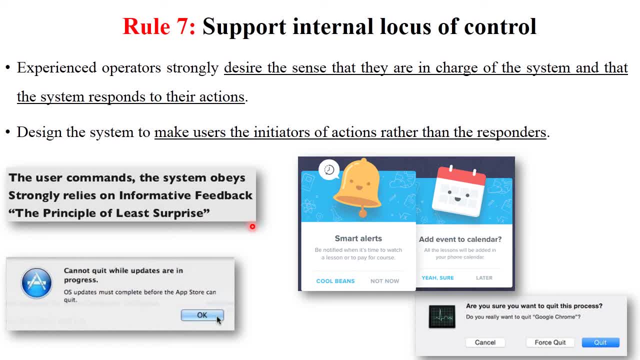 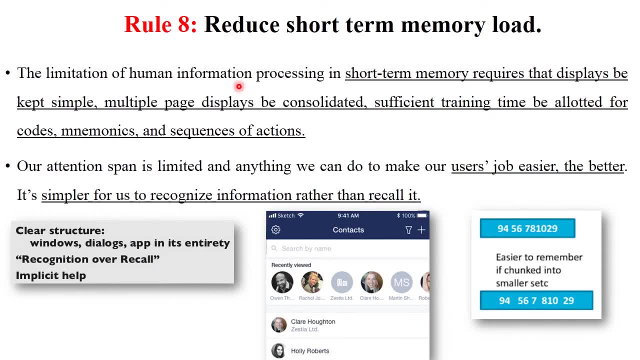 surprise, right? so, as per the user's command, the particular design or particular system will be work clear. next, the last golden rule is reduce short-term memory load. we will learn different types of memory- short-term memory, long-term memory- in the previous videos, right? so this principle is.